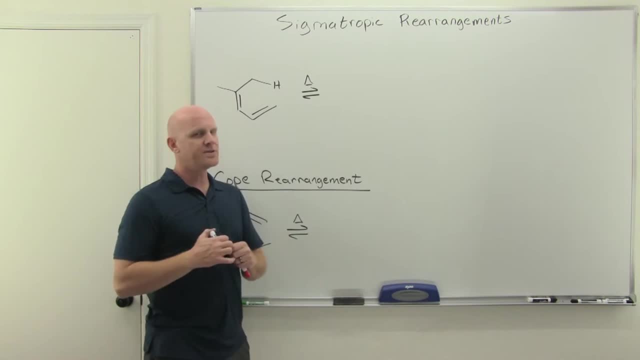 sigmatropic rearrangement And, where those occur, is going to lead to some numerical notation, as we'll see here. So come, take a look at the motion of electrons in this one. So we're going to have the cyclic movement of six electrons, just like so, And, if you notice, by moving around in a ring like this: 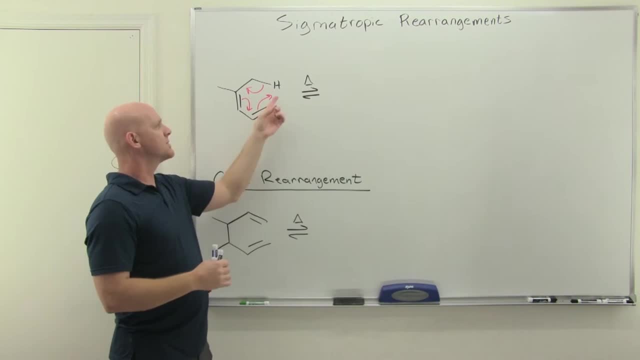 every atom in that six-membered system- I can't really call it a ring, but a quasi-ring, if you will- every atom there is going to both be losing a bond and gaining a bond, so that we don't violate the octet rule in any way, shape or form. So we are forming a new sigma bond right here And then 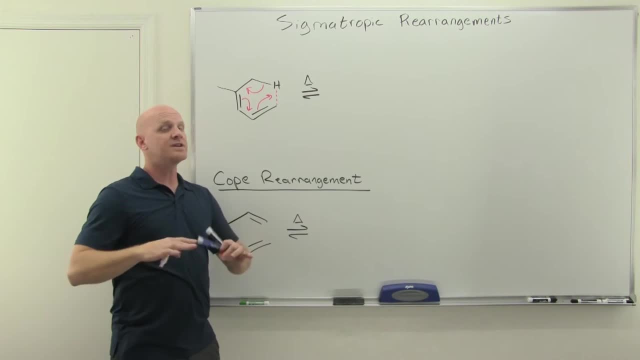 we're breaking a sigma bond right here, And where those are located in relation to each other, there's a numerical system in which we'll name, or at least signify, our sigmatropic rearrangement. Now I want to draw the transition state in this case. So, because the transition state is going to 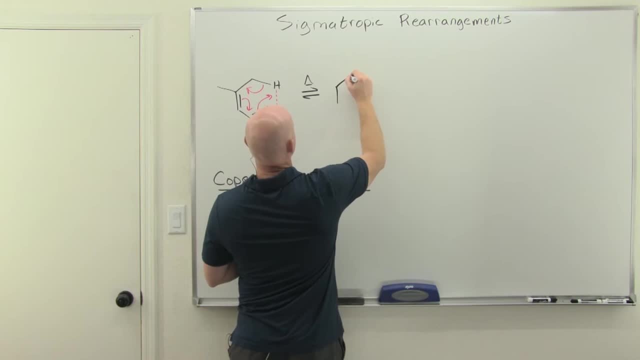 look somewhat like a six-membered ring. So if we take a look here, we've got a partial bond here that's breaking And I'm going to draw that in blue So. and then we've got a partial bond that I really put as a partial bond here, but technically it's a partial bond in the transition state. 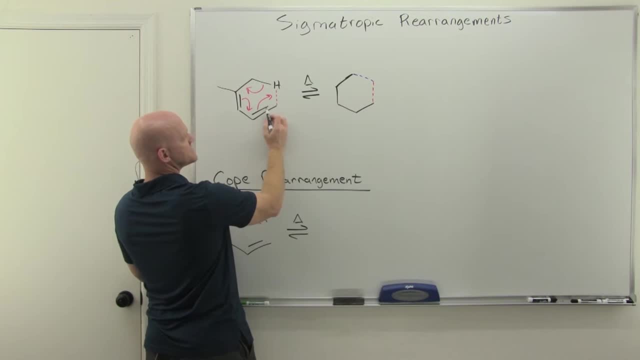 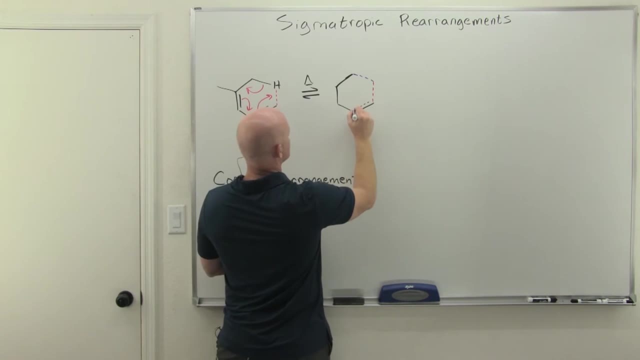 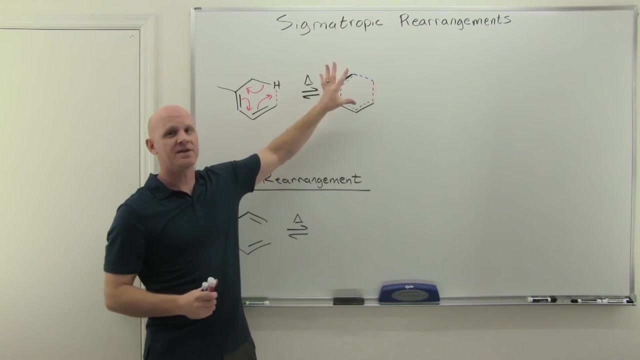 All right. But then we also got a partial pi bond for this, one that's breaking right here. So we got a partial bond for one that's forming, one that's breaking and one that's forming in all three of those locations, And so you can see this complete ring of partial bonds in the transition state. So 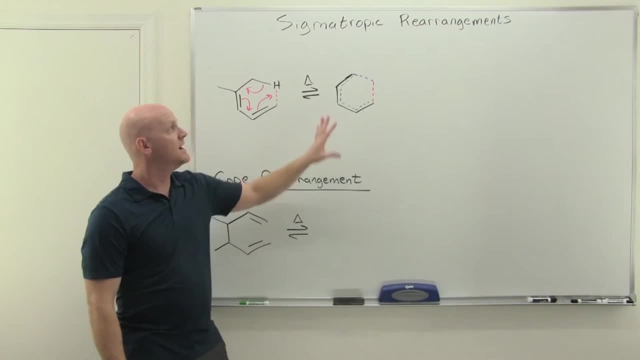 our reactant is not a ring and our product is not going to be a ring in a second either, But in the transition state we have a ring-like structure. So, just due to all the partial bonds that are forming and breaking, And again the bonds that are forming or breaking that are sigma bonds- these are all pi but the. 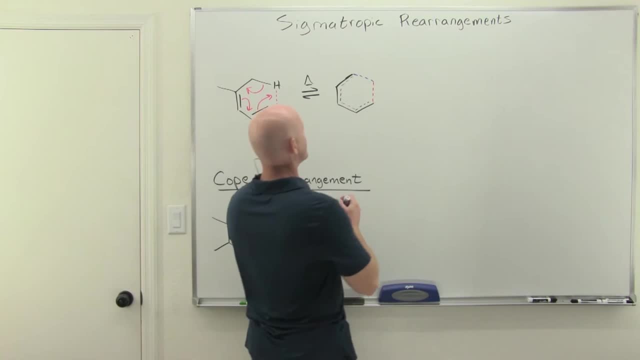 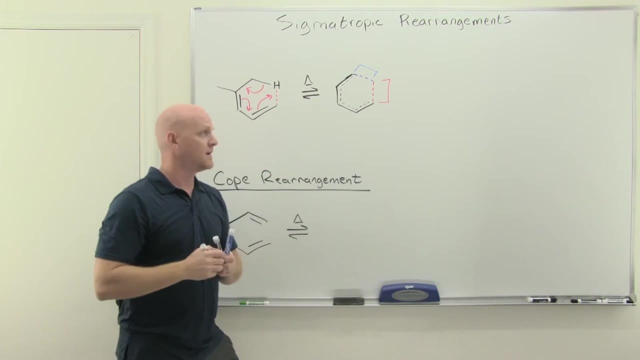 sigma. I signified those in blue and red because those are going to be useful to us. In fact, I want to really highlight that a little bit better, So I'll do it like so, just so we can highlight where those new bonds were broken and formed. All right, So this is kind of what's going on Now. one thing: 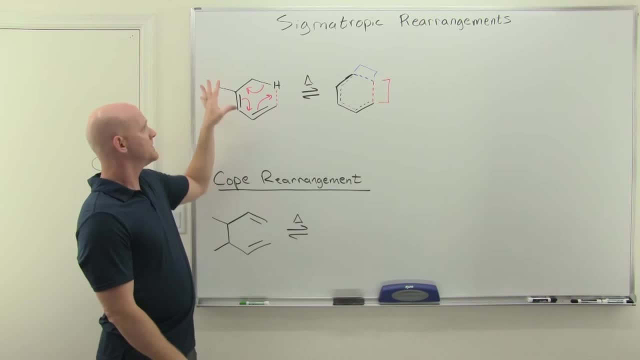 you should know, when you're trying to predict the product in a sigmatropic rearrangement, if your reactant is not drawn in such a way that you can kind of see the five-sixths of a six-membered ring. So it looks like the way I've drawn it. 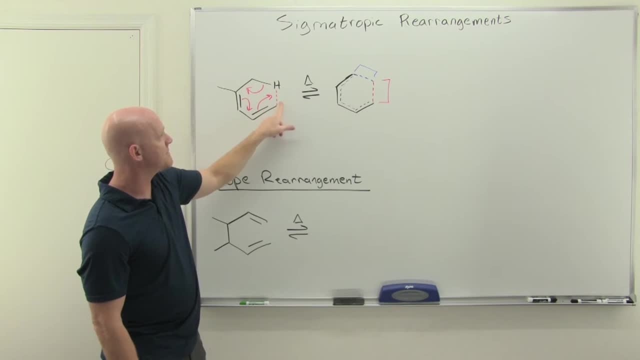 here it looks like almost like a six-membered ring, like a cyclohexane, just that bond was missing. In fact I'm going to take it right back off, So as we've drawn it in the transition state where it really belongs. but it's five parts of a six-membered ring And obviously this is just a. 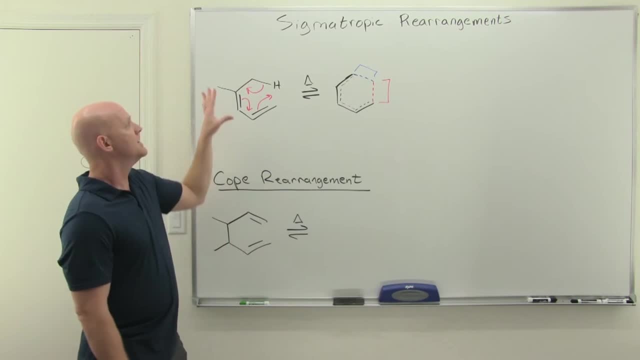 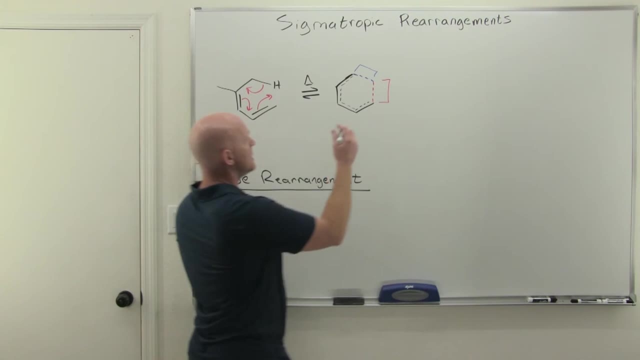 straight chain and I can draw it out as a straight chain. But if you're trying to predict the product, you're going to want to redraw your reactant so that you've got five-sixths of a six-membered ring, so to speak. And so if we keep going with this and go to the final product here, 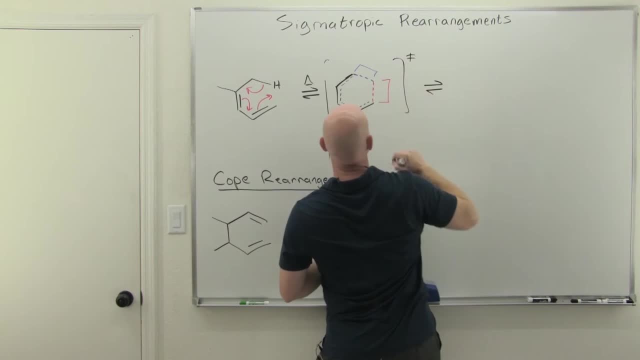 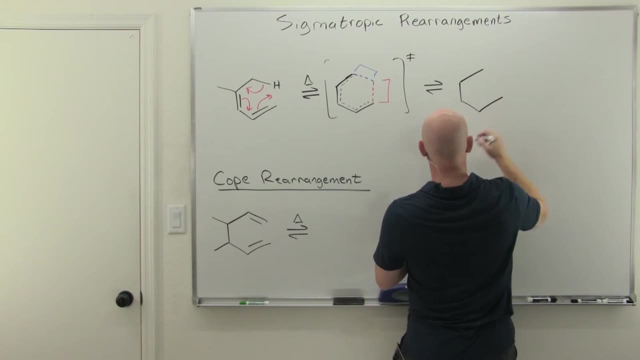 so, and again, this is technically the transition state. So now we're going to have a new bond to the hydrogen, right like so that's forming right here, but then this bond of the hydrogen is now broken. but we're going to have pi electrons both here and here and still have that methyl group out there. 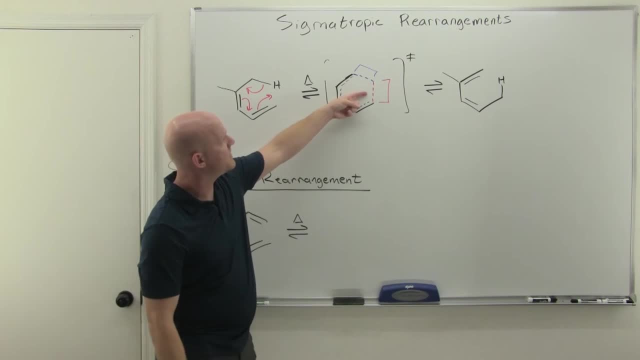 So there's our product. So again, we've formed a new sigma bond in red in the transition state and we're breaking one in the transition state in blue. And again, how those are related to each other is how we're going to. 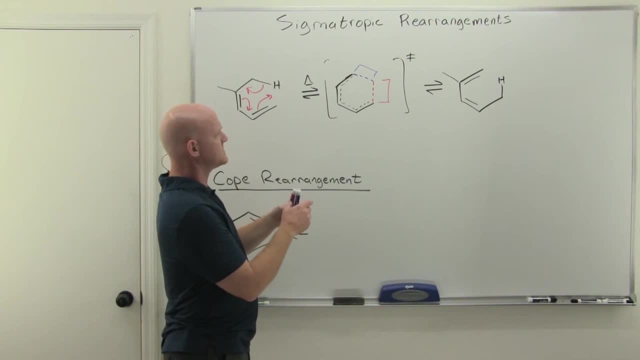 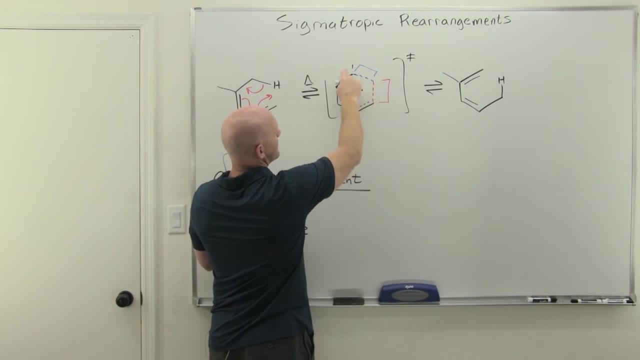 signify numerically where this rearrangement took place. And so what you want to do is actually count around from sigma bond to sigma bond, starting with the end atom. So let's say, I start with this as number one right here, and I want to count all the way over to this atom right here. 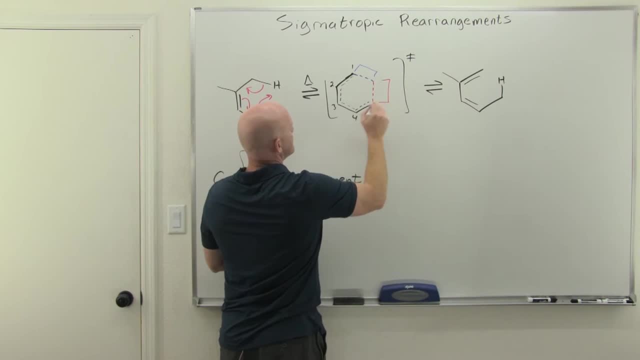 And so one, two, three, four, five, So that's half of the numbering system. Now I want to go to the other side of one of the sigma bonds, and that just happens to also be the other side of this sigma bond. So, and I want to count how far it takes to get from this end of this sigma bond. 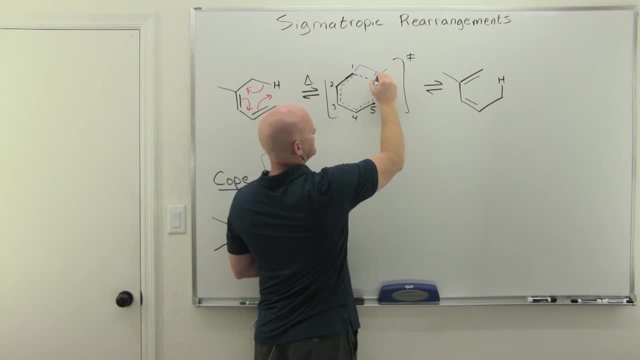 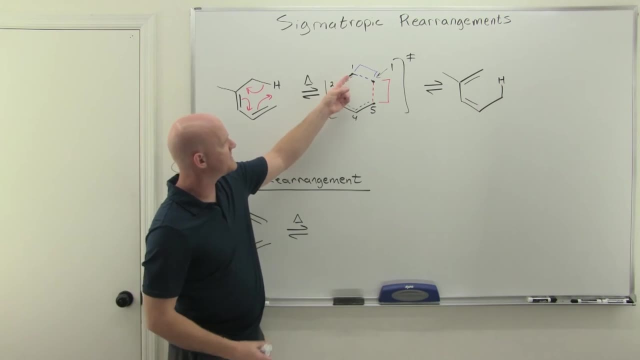 to this end of this sigma bond. Well, it just takes that one atom, And so most of the time you're going to see more than one in most cases. So, but you just want to identify the ends of the sigma bonds and count around on one side, but also count around the other side, And so 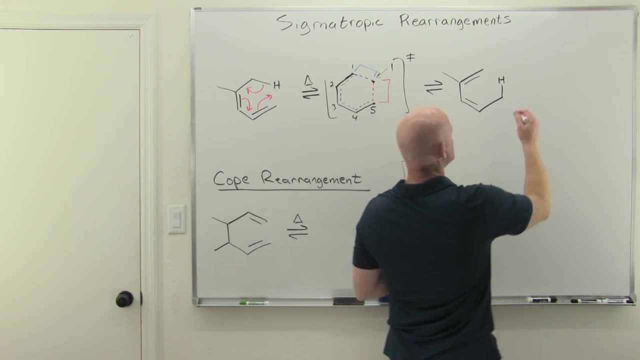 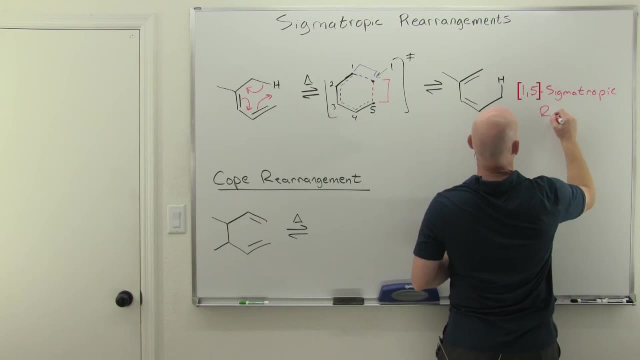 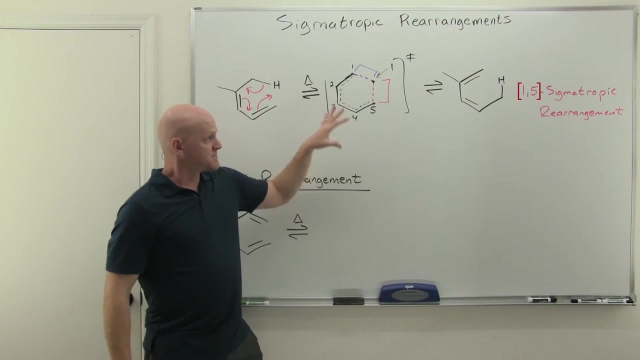 we got one there, we've got five here and this is a one five sigma tropic rearrangement. Okay, Cool. Now this is probably not the best example to start with, as far as that numerical notation goes, and seeing the one and the five it'll be a little easier to see on this next example. So 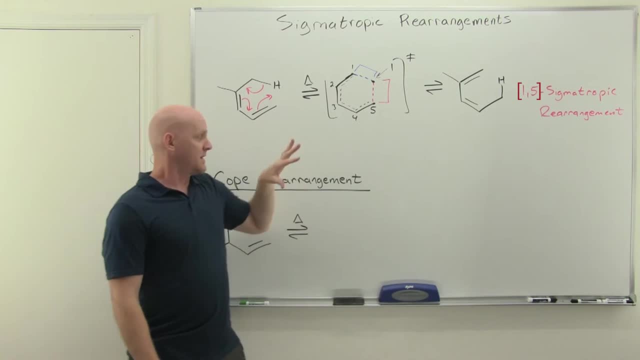 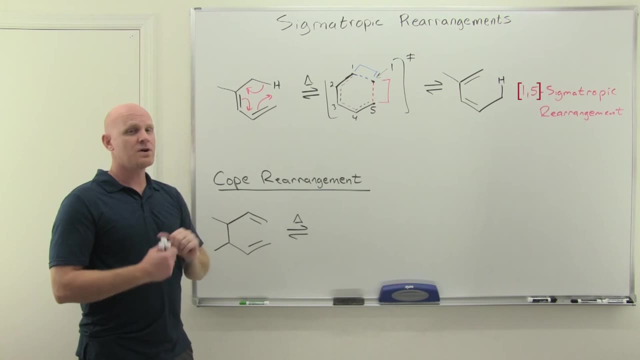 but for every other respect, this is probably the best example to start with. So because the rest of the reactions are going to actually have special names. So this next one is called the cope rearrangement, And again, all of these are going to involve one sigma bond being broken. 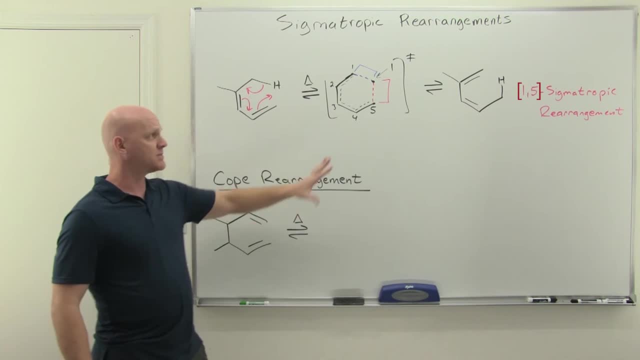 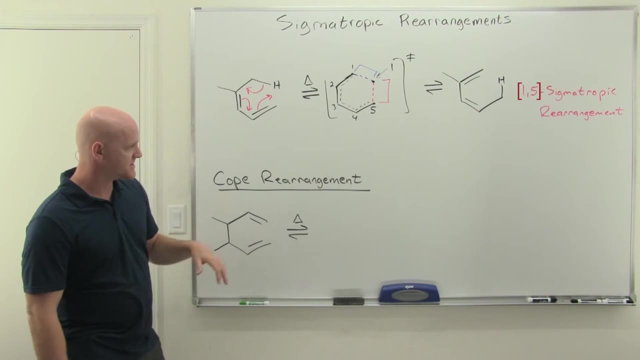 one being formed, a six membered ring like transition state. I probably won't draw the transition state again. I'll probably just signify where we're actually going and breaking the sigma bonds on the reactant so we can get the numerical notation. but I did want you to see it once, So but in this case they're going to get special names here: The. 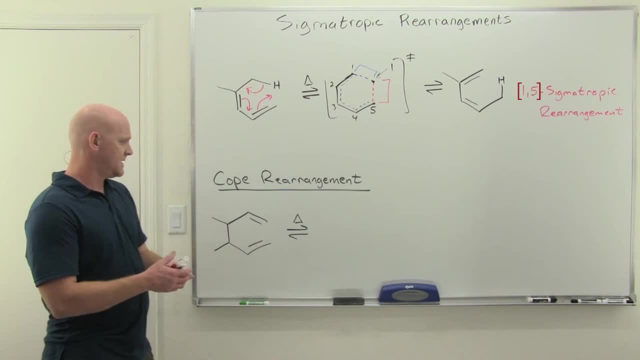 cope rearrangement turns out as a three, three sigma tropic rearrangement by definition, And so in this case we look at the cyclic movement of electrons. here We're going to form a new sigma bond right here, and then we're going to break one right here. So in fact I'm going to 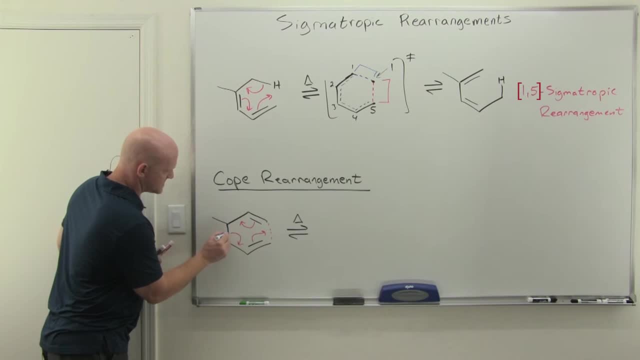 erase that and redraw it in blue, just so we can kind of keep track of it. And so once again we've got the bond- sigma bond we're breaking there and the sigma bond we're forming there, And rather than draw the transition state at all, 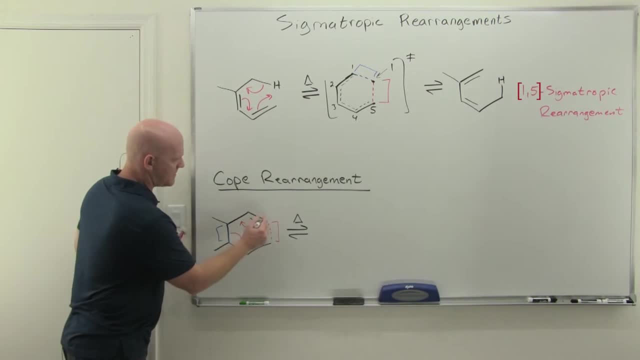 I just want to show you how to identify it on the reactant then. So I just want to say, how many atoms does it take to go from here to here and from here to here? And so we got one, two, three, one, two, three- It doesn't really matter which way you number it- and stuff like. 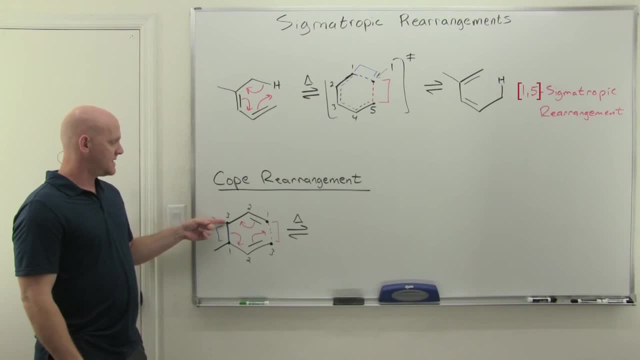 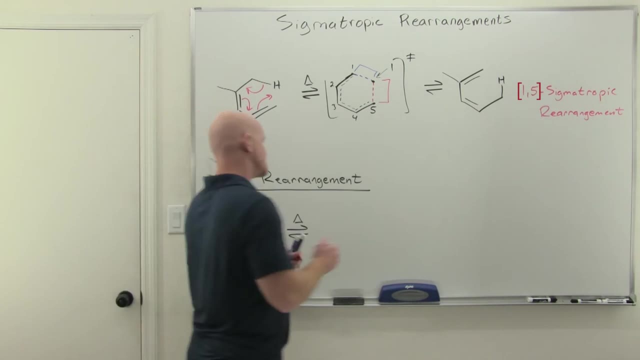 this So, but from one end of the sigma bond you're forming, to the nearest end of the sigma bond you're breaking. it's three atoms included, So, and same thing on the other side, And that's why we're going to refer to this as a three, three sigmatropic rearrangement. 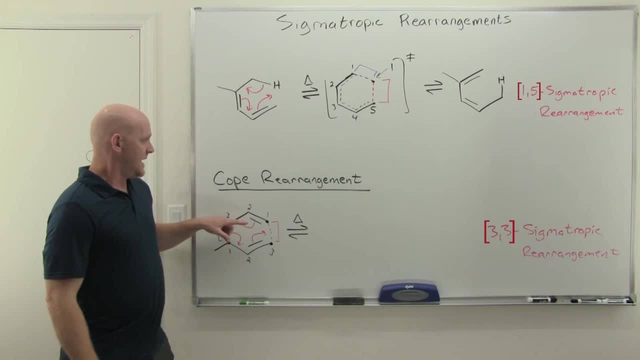 Cool, And again, that's what a cope rearrangement is, And so it turns out there's also going to be what's called a Claisen rearrangement in the next example, And a Claisen rearrangement turns out is also a three, three sigmatropic rearrangement. So I just want to make 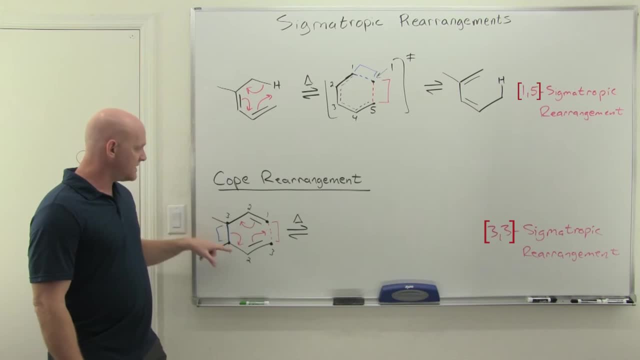 sure you realize what the difference is. So the Claisen is going to involve one of these six atoms being an oxygen, So it'll be an ether reactant, Whereas the cope is specifically if they are all carbon atoms. So that's just to keep the difference there from the get-go. 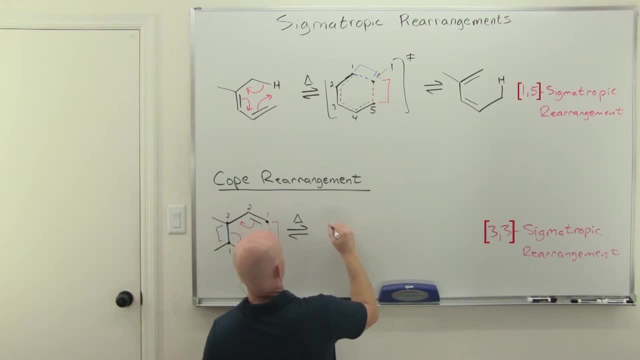 All right, So let's draw our product as well, And in this case we are going to have a new bond right there. So we're also going to have a pi bond here, a pi bond here, and that's it actually. 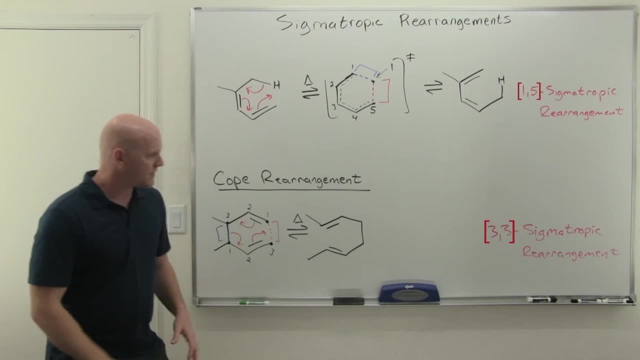 So there's our new product Now, most of the time. so you're going to be able to actually, in these equilibrium, you're actually going to get a mixture of both your reactant and your product, And often you can predict which is going to. 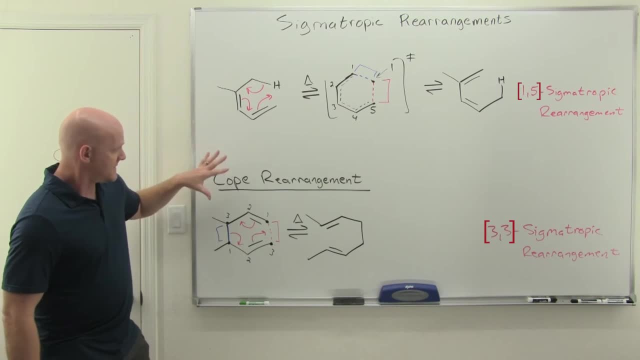 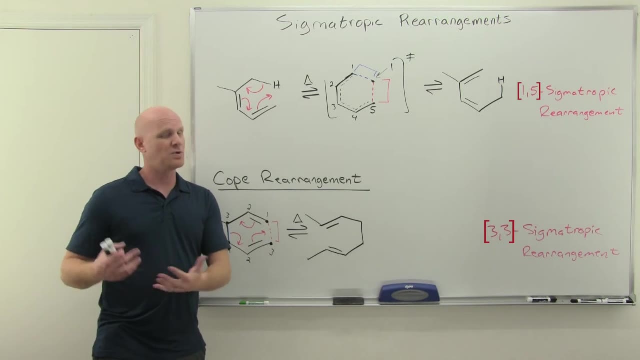 predominate in your product mixture. So in this case it's going to be about the more substituted alkene. In other cases it might actually be about having a more stable double bond, for example, or something else in a unique example we'll talk about later as well. 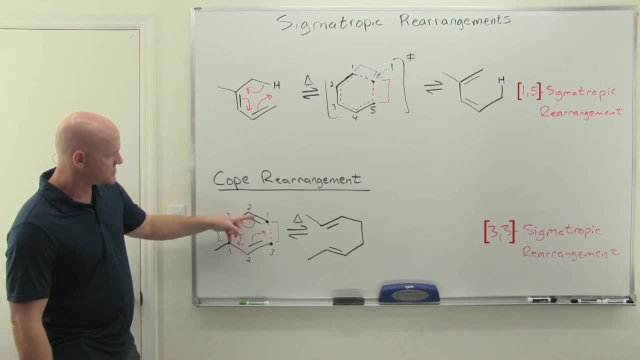 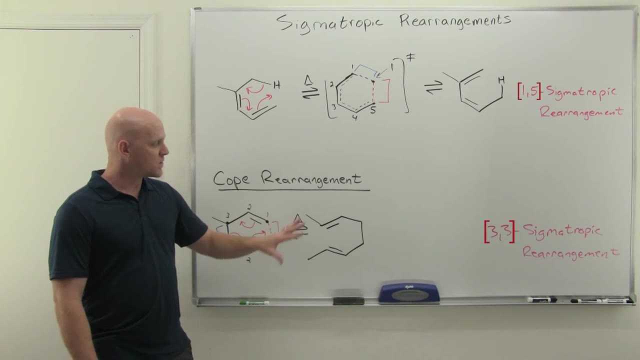 So, but in this case really is going to come down to the more substituted alkene. And if we look at the two alkenes in the reactant, here these are both monosubstituted, Here they're both disubstituted. And we learned earlier, the more substrate alkene is, the more stable alkene And 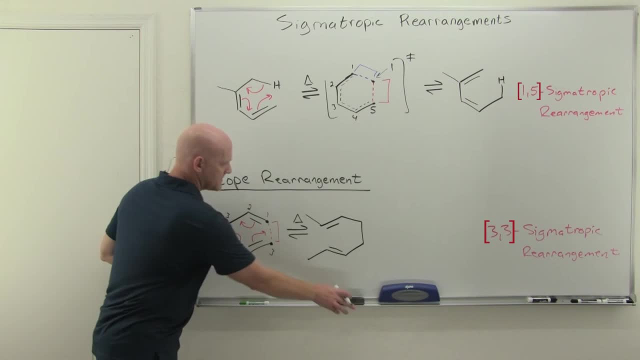 because this product is more stable, so it is going to be favored in the equilibrium, And so we could redraw the equilibrium arrow to reflect that as well. And so sometimes you'll be asked not only to predict the product, but then also to predict which is favored in the equilibrium. 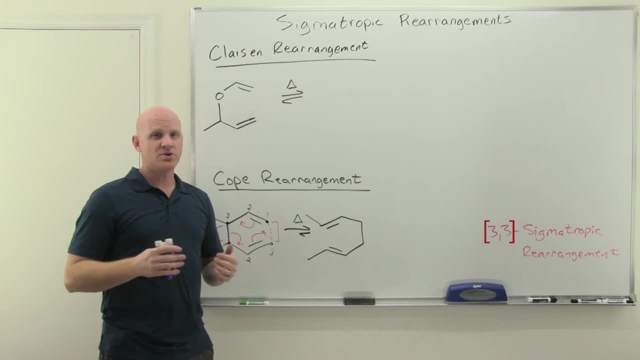 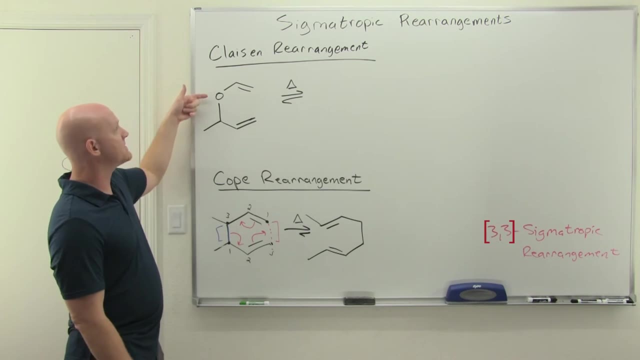 the reactant or the product. All right. So in the Claisen rearrangement here it's also going to be a 3,3-sigmatropic rearrangement first off. But the big difference is we're going to have an oxygen in our almost ring-like structure, our five-sixths of a. 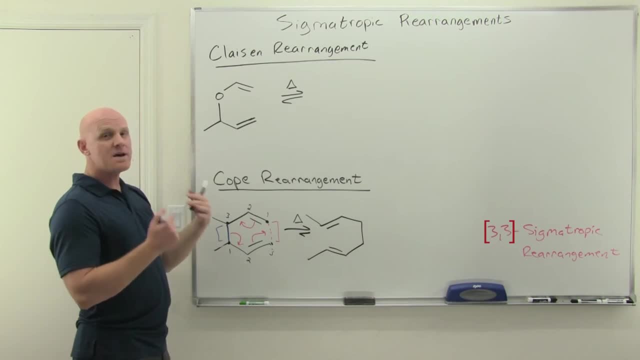 ring. So this is going to be an ether reactant And typically the way it works. for your typical Claisen, we're going to see an atypical one in a sec. but for your typical Claisen you're going to have a vinyl group, a simple carbon-carbon double bond on one side and then an allyl group. 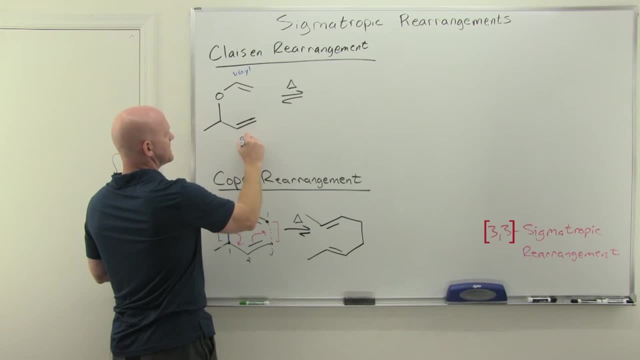 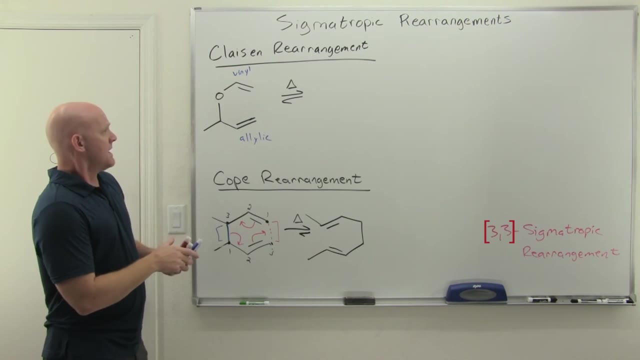 so three carbons, where the allylic carbon is attached to the other side of the ether. So you're going to have a vinyl-allylic or vinylic-allylic ether. So as your reactant, All right, We're still going to have the cyclic movement. 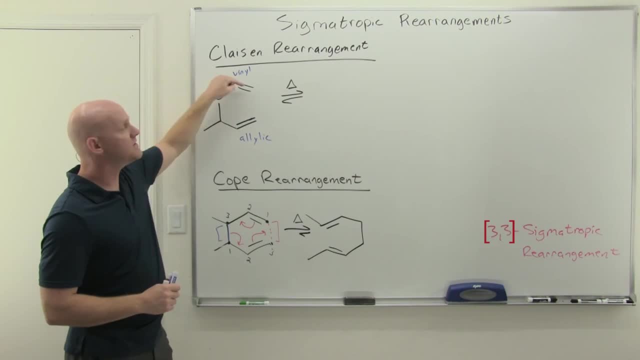 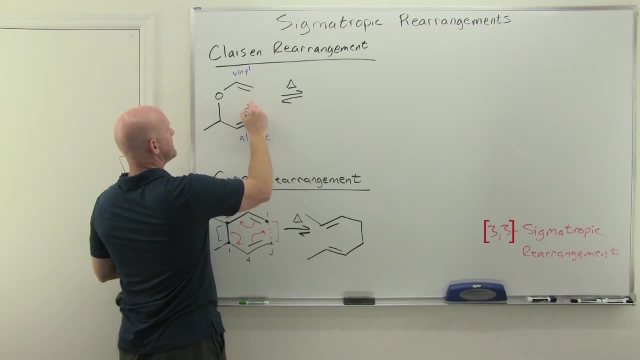 of electrons. And again, if your reactant isn't drawn in such a way that you can almost see the six-membered ring, then you're going to want to redraw it into that conformation. We get the cyclic motion of electrons here. We're going to form a new sigma bond right here. 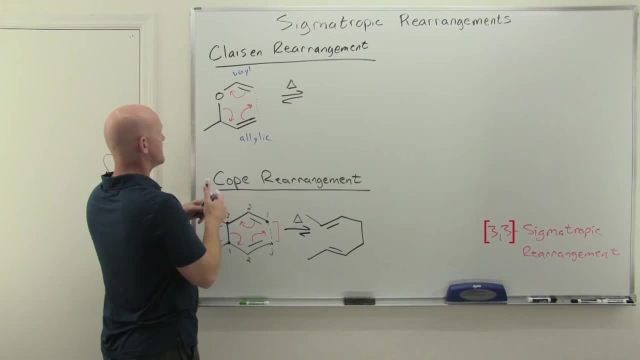 So we can see that we're breaking the sigma bond on the opposite side. So I'm going to erase that and redraw it in blue, just so we can see that it's a 3,3-sigmatropic rearrangement once again a little more easily. So there's the bond we're breaking. Here's the sigma bond. 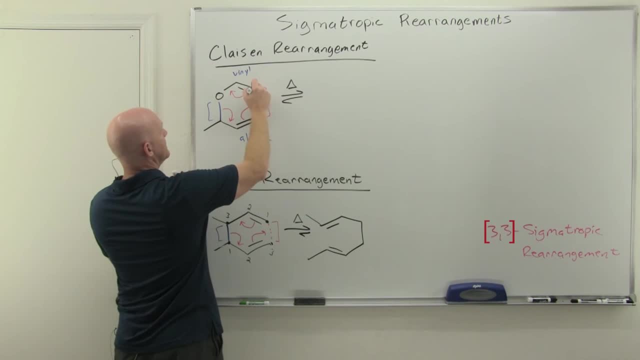 That's what we're forming, And so, once again, you're going to get a From this atom to the oxygen, One, two, three, And on this side, from this atom to then this atom, One, two, three. 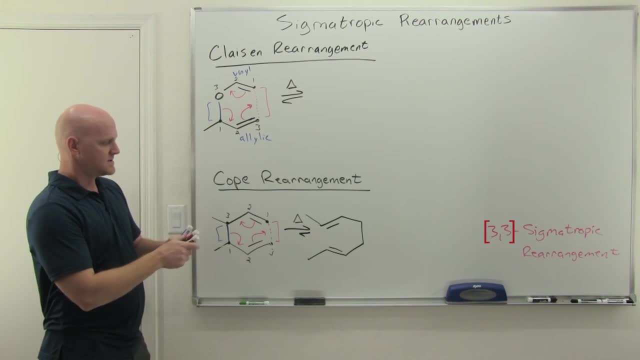 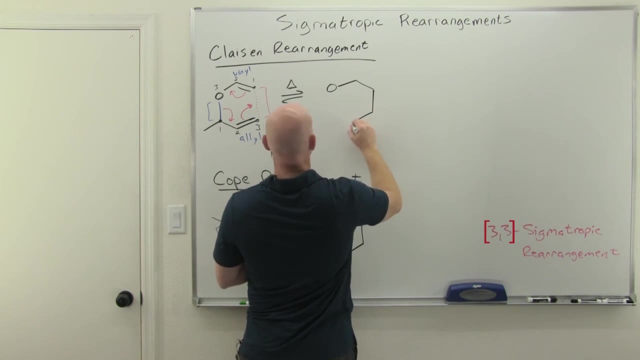 And again, that's what makes it a 3,3-sigmatropic rearrangement. So if I take a look at that product now, So we've formed a new sigma bond here. We broke this sigma bond right here. Now we're going to have a carbon oxygen double bond. 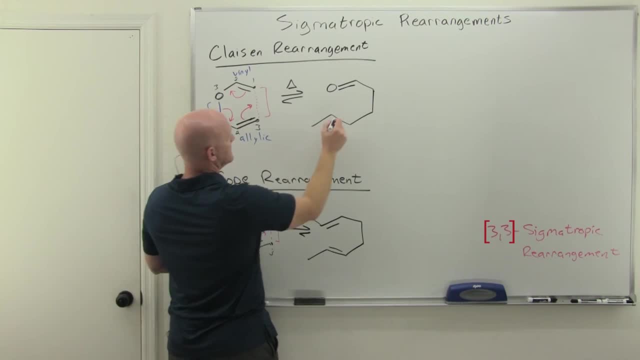 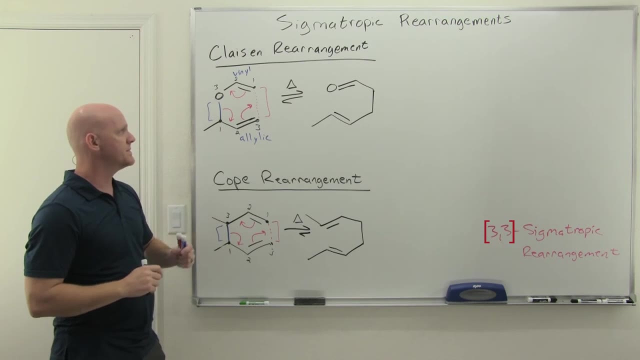 right there as well. we're also going to have a pi bond in this location as well, and there's your product. so, and again we can talk about which of these actually gets favored in the equilibrium. but here it's not about having a more substituted alkene, because here we've got two alkenes, whereas 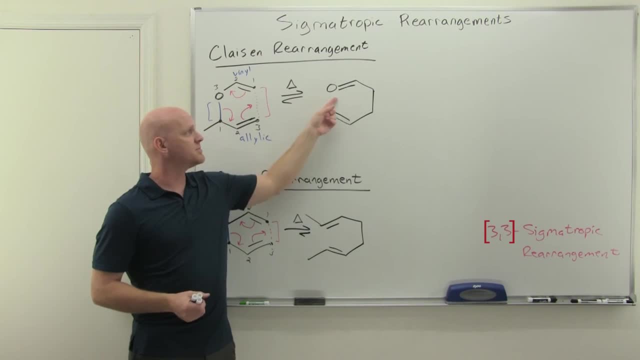 here we've got one alkene and then one carbonyl, and that carbon oxygen double bond, with oxygen being more electronegative, so one. this is a stronger and shorter bond, so but also with the more electronegative oxygen, for other reasons as well being electronegative, it actually lowers the 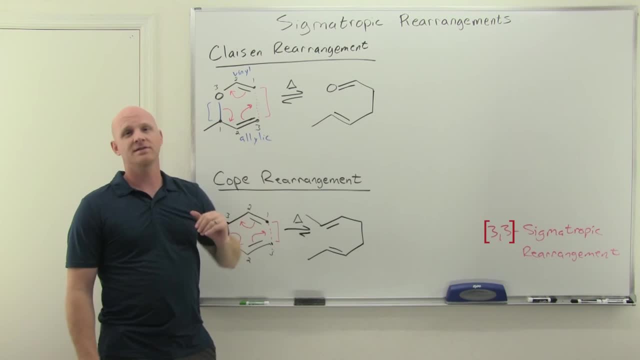 energy. so it's a shorter bond, it's a stronger bond, it's a lower energy bond- all those things kind of being somewhat synonymous so- but it is a lower energy bond and so that's why this ends up being the more stable product. so more stable to have a carbon oxygen double bond than a carbon. 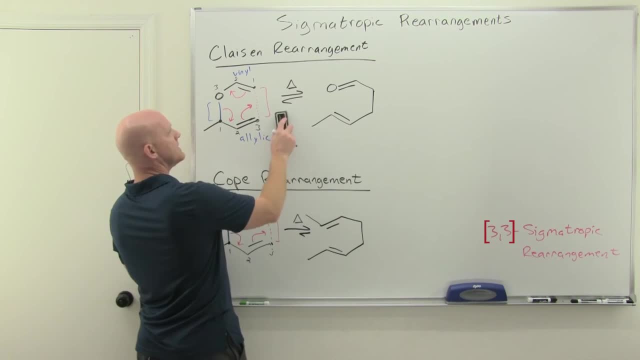 carbon double bond, and so if we redraw our equilibrium arrows here once again in this example, it favors our product. cool, technically this is an aldehyde and if you form an aldehyde, good practice to probably draw in you the aldehyde hydrogen, the one time we kind of find it necessary in organic chemistry to draw. 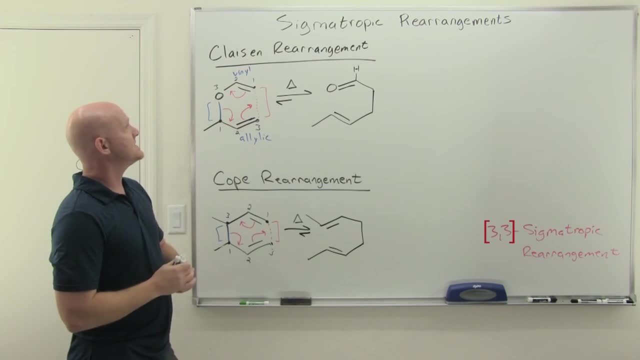 a hydrogen bond into a carbon atom. okay, so that's your typical clays in, and just want to show you the similarities and differences with the cope again. this is also a 3-3 signotropic rearrangement, but now i want to show you a little less typical clays in as well, so we'll get rid of the cope here. 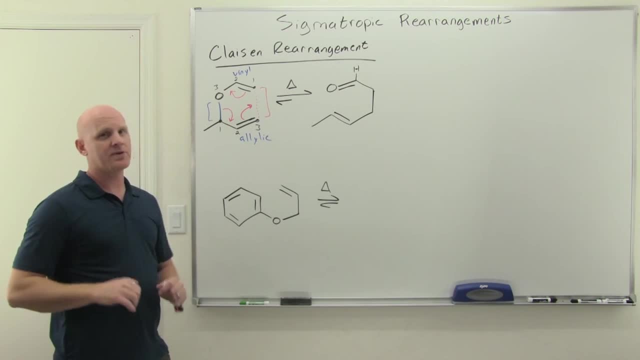 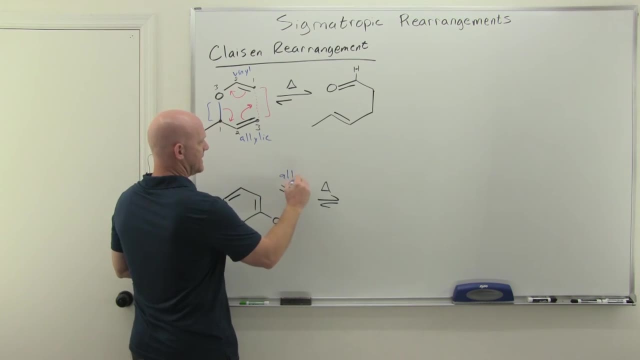 all right, so your other, less typical clays in condensation. instead of having a vinylic allelic ether, you're going to still have an allelic condensation, so you're going to have a vinylic. you're going to have an allelic on one side, but instead of vinylic you're going to have a. 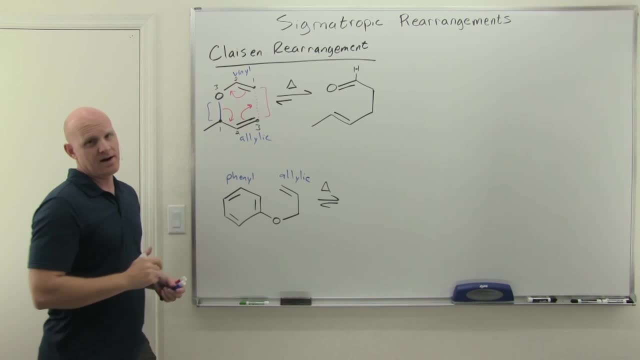 phenyl ether on the other side. so it's a phenyl allelic ether in this less typical instance. but again, you want to draw this in such a way that you can almost see the six-membered ring here. still do the cyclic movement of electrons here. 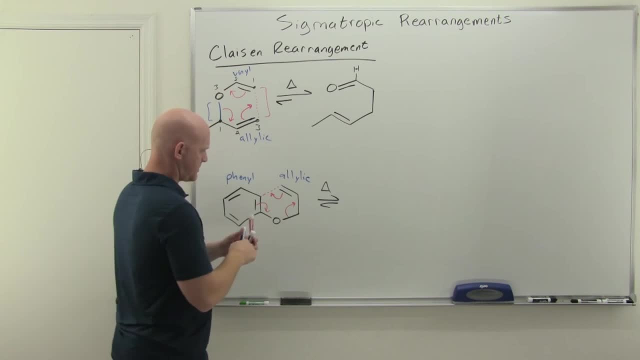 so forming a new sigma bond right there, breaking a sigma bond right there, and you can quickly see that it's a one, two, three. one, two, three, three, three. sigmatropic rearrangement still, and since oxygen's involved, that's what makes it a clays in. 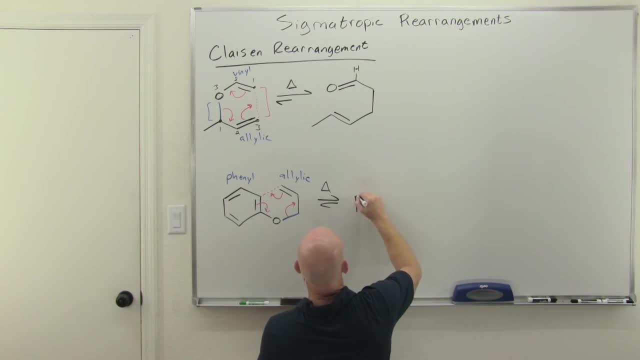 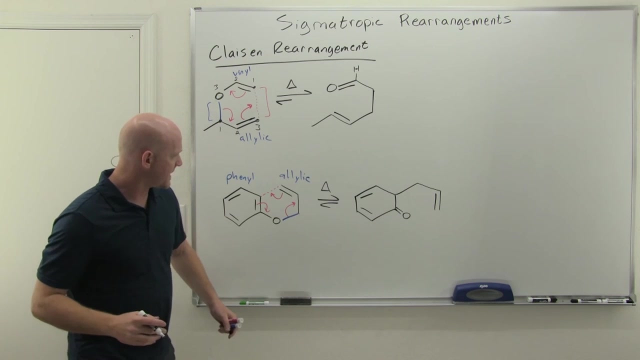 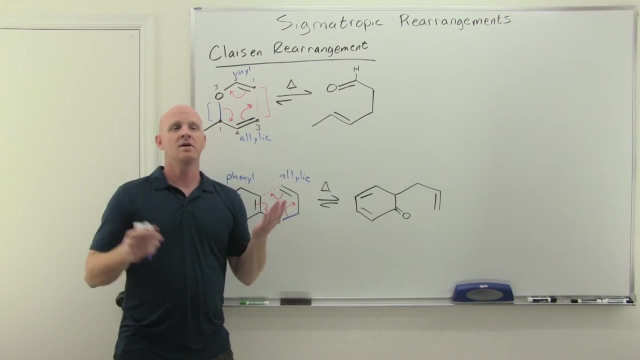 so if we draw our product this time- all right, see if i forgot anything here. note looks great, all right. so there's our product. in this case, instead of being an aldehyde, it is a ketone instead. great well, we didn't consider this possibility before, but we're going to consider it now, so 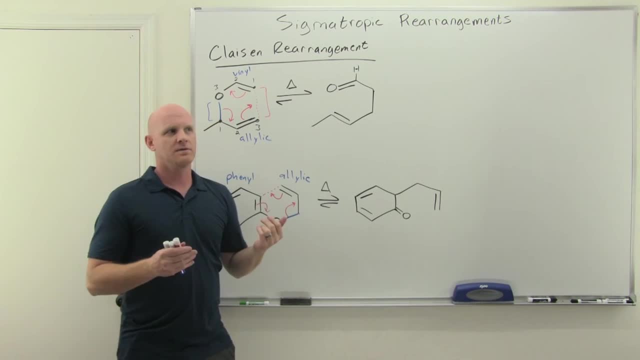 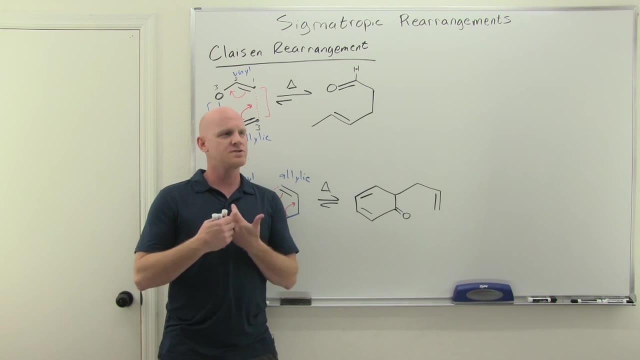 it turns out whenever you form an aldehyde or a ketone, so you're typically going to have both keto and enol forms present, but in most of the cases, we learn that the keto form is usually much more stable, and so usually the keto form heavily predominates. so, however, uh, and that's why we didn't- 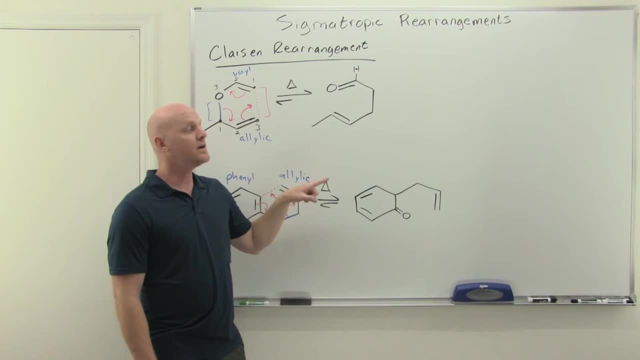 even consider up here. we just drew the aldehyde and we're done with it. we didn't have to worry about the enol, but here it turns out as a special case. so in this one instance the enol is actually going to be very stable. in fact, it'll be more stable than this corresponding keto form, which 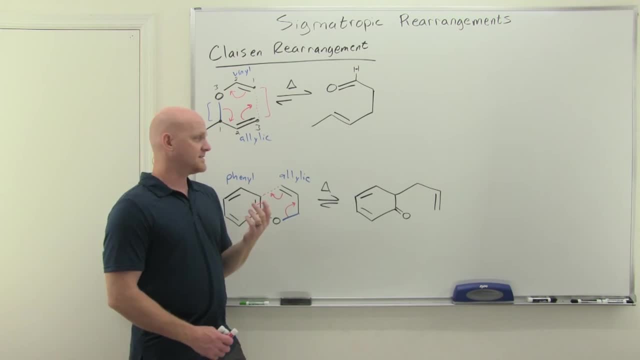 is why this is not your actual final product. so- and it's not normally something we check for, but now that you've seen this version of the clazen, when you have a fennel allylic ether, so you're not done. once you form your ketone product, you got to go one further step, and so, if we take a look at 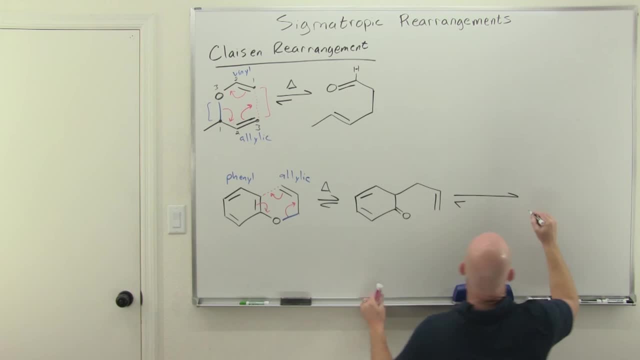 the enol form here, and so notice, now we're going to have an alcohol and an alkene, and the big thing is not just an enol like an alkene, you know, but it's a phenol, so it's got a complete benzene ring. 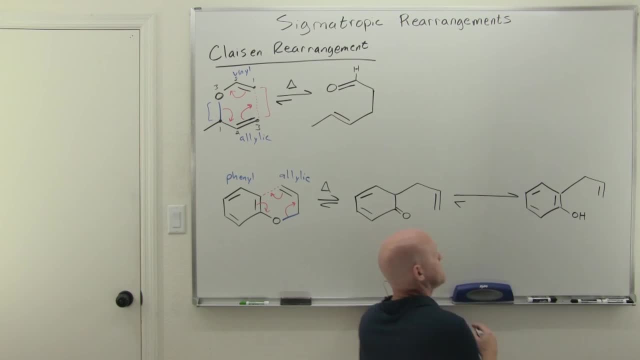 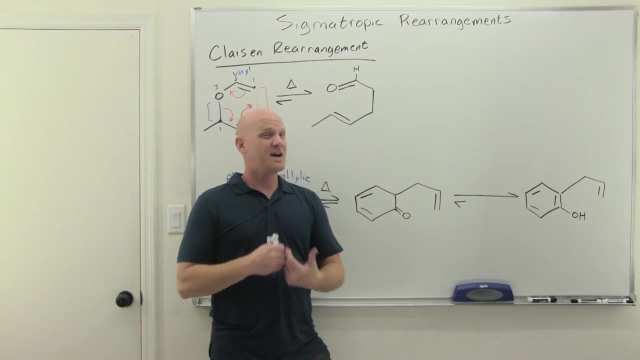 which is aromatic. so, and that's what's actually driving the stability of this reaction. so, with it being aromatic, we're going to talk about aromatic compounds in the next chapter, but suffice it to say they've been designed to support the- the cyclosphate reaction. now.